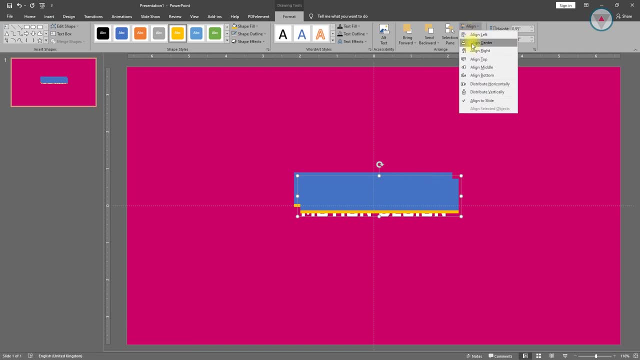 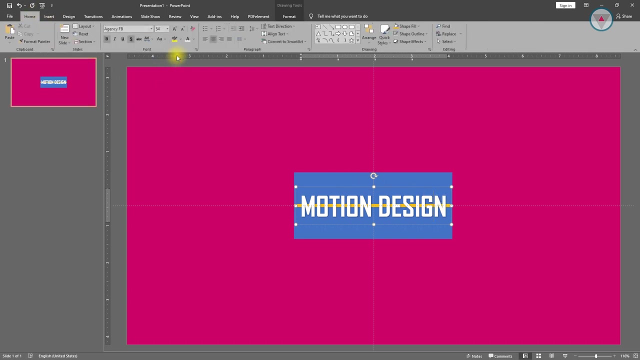 Change its alignment: align center And rotate it. Flip vertically, Drag it down And select this two group by holding down the ctrl key And send them to back. Now we need to separate this text into two object, So change its alignment: align left. 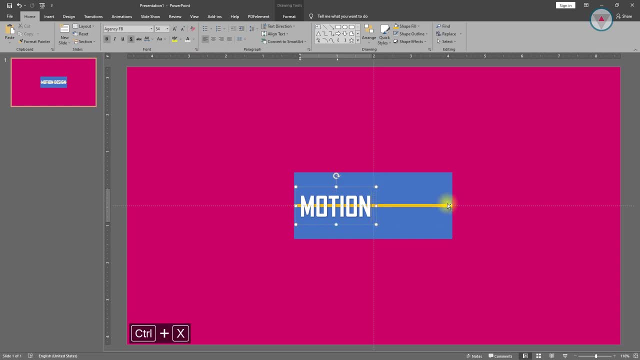 And select design. Cut it by pressing ctrl plus X. Select align right And duplicate this motion by pressing ctrl plus D And drag it in the right side And paste the design by pressing ctrl plus V. Bring this two group in center. 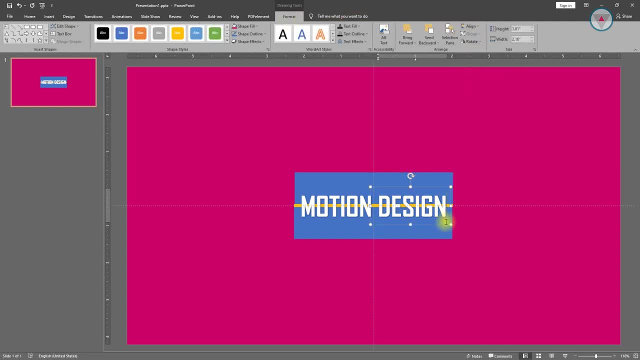 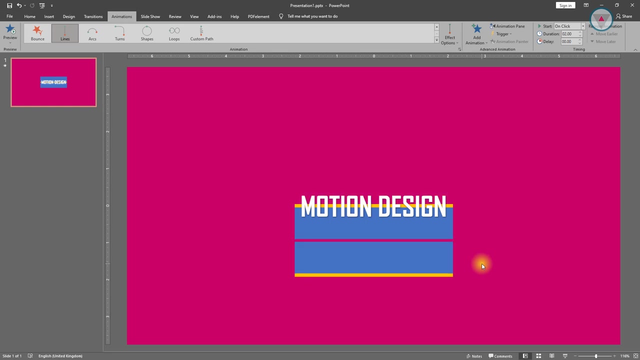 So change their alignment align center. Now it's time to animate. Select this group And apply the lines animation. We need to apply the lines animation again. Go into the animation pane And select this animation. Change its path direction to up. 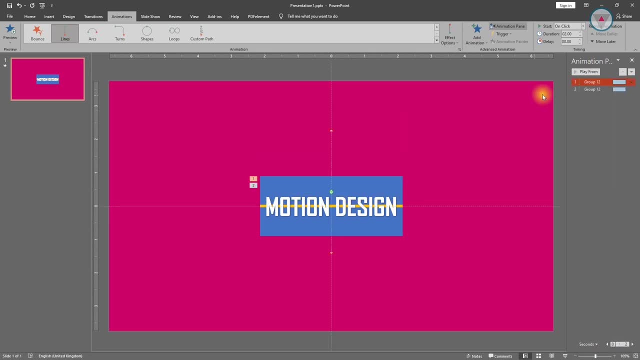 And select this animation, also Change its path direction to up And reverse too. After doing this, we need to apply the lines animation on this group. Apply the lines animation again, Select this animation And change its path direction to reverse. Then select all of this animation by pressing ctrl plus A. 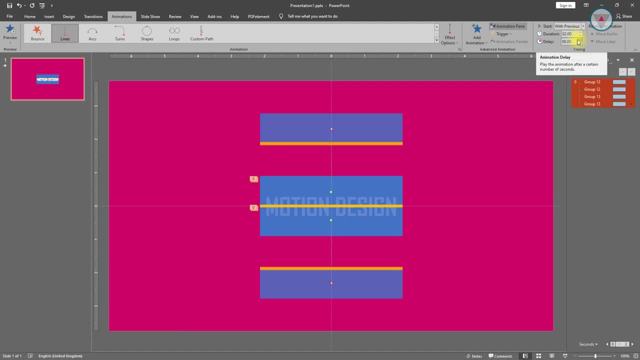 And select start with previous Duration will be 0.75 second. Then select this animation and this animation By holding the ctrl key And increase their delay 0.75 second. It's too fast. Delay will be 1.25 seconds. 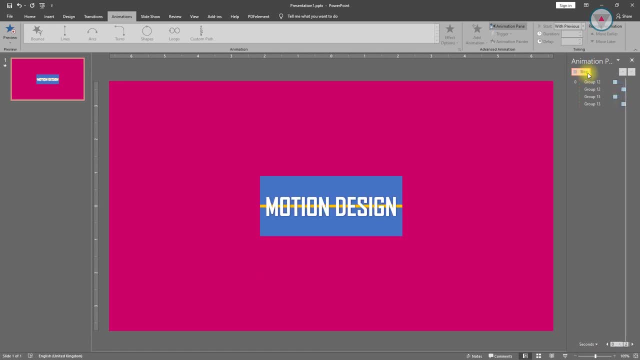 Perfect. Select this starting point And drag it down. Select this end point, too, And drag it down also. After doing this, we need to bring this starting point And this end point too, up. Let's see the preview of this animation. 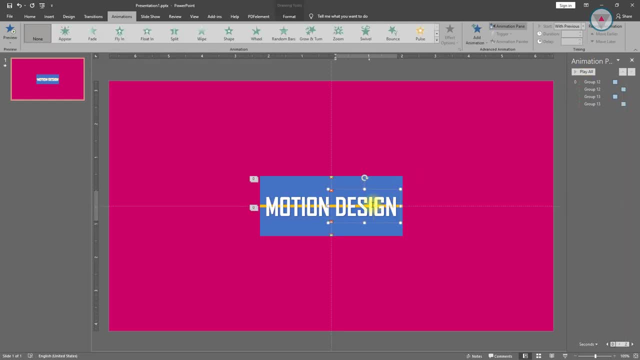 Perfect. Now we need to apply the lines animation on this two text. Select this text And apply the lines animation. Apply the lines animation again. Then select this animation And change its path direction to up And reverse too. Then select this animation. 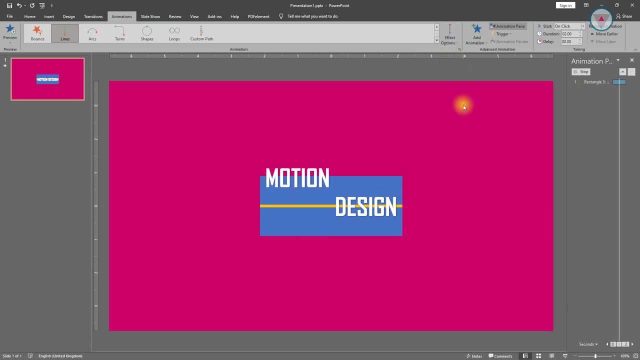 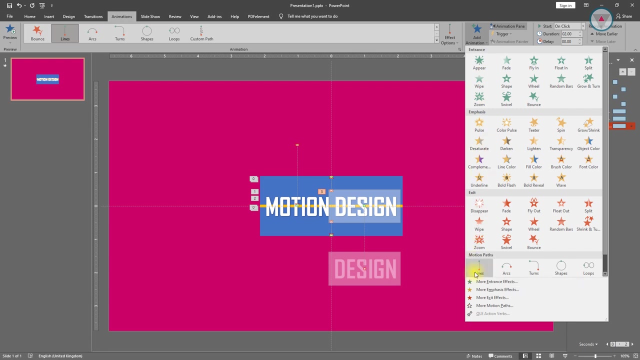 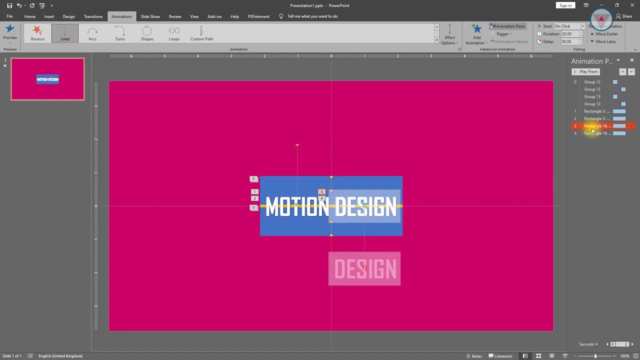 And change its path direction to up. After doing this, Select this text And apply the lines animation. Apply the lines animation again. Then select this animation And change its path direction to reverse. After doing this, Select this last four animation. 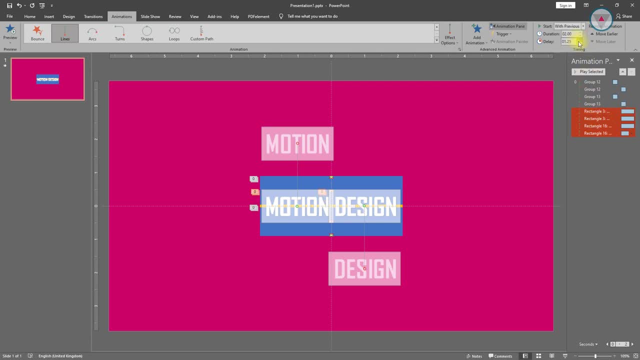 And select start with previous. Delay will be 0. And duration will be 0.75 second. Select this animation And this animation And increase their delay 1.25 second. Let's see the preview: Perfect After doing this. 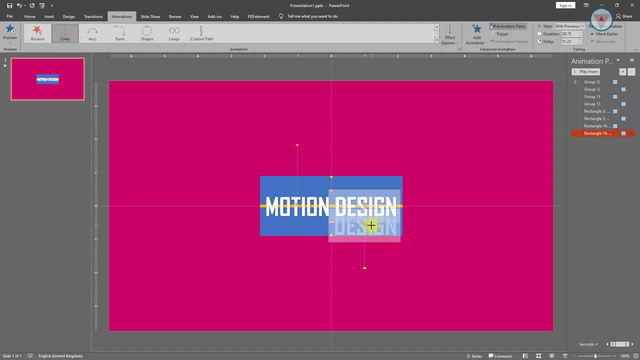 Drag this end point in here And drag this starting point too. Then select this end point And drag it down. Select this starting point too, And drag it down also. Let's play the animation, Open this television and Let's see the edit. 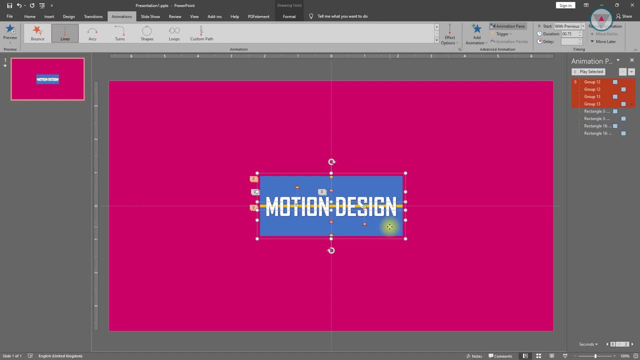 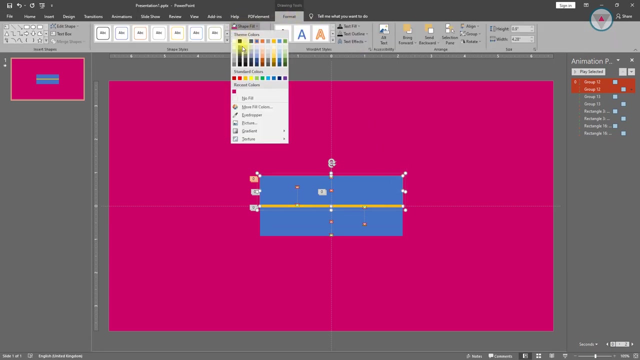 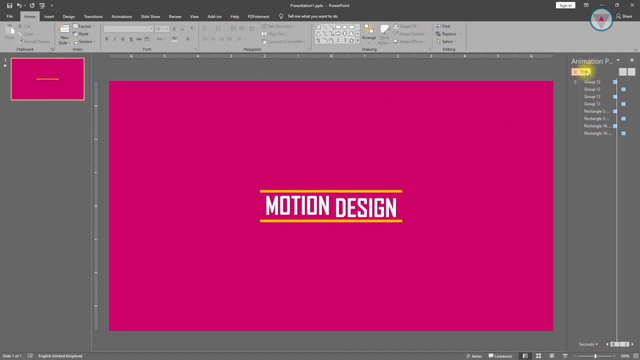 And drag this end point And drag it down also, Then its same. Then press this click And create chapter file in this editor Here. make the folder Now. open this bug And then disable here. Double click in that tab. 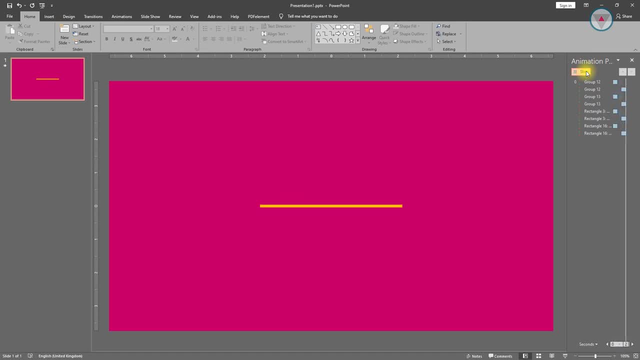 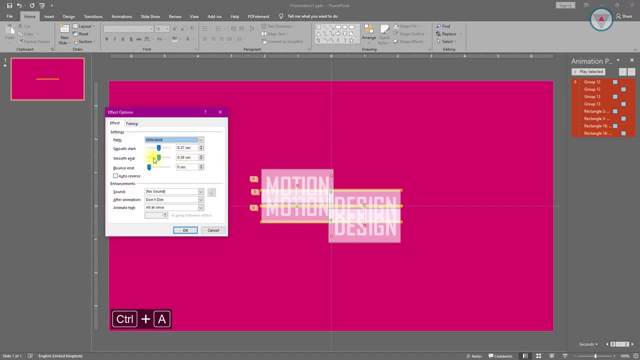 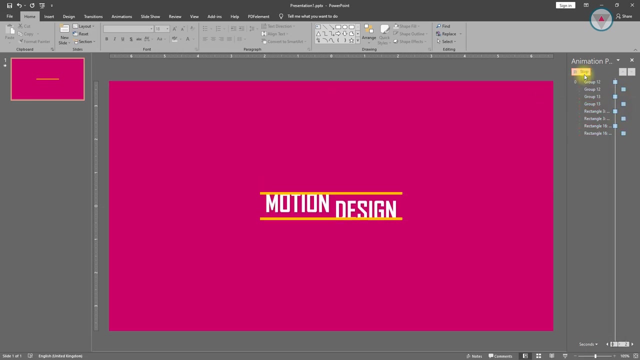 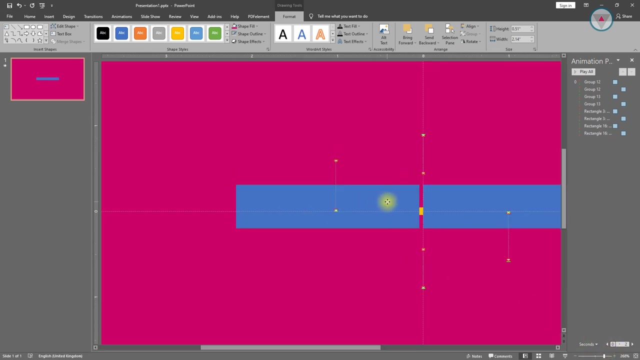 select all of this animation and, going to the effect option, increase the smooth and duration. let's see the preview perfect. now we need to take a rectangle shape and drag it in here. change its outline color to no color, duplicate it by pressing ctrl plus D and drag it into left side. click here to zoom in the slide bring. 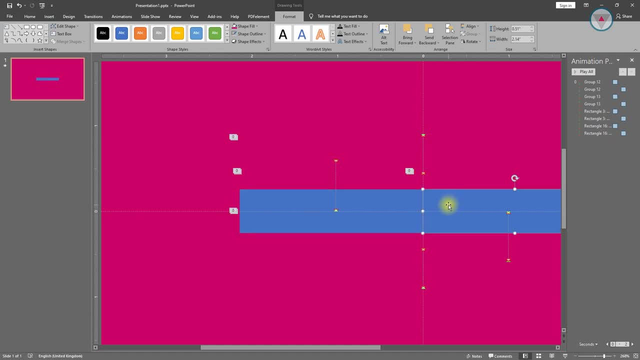 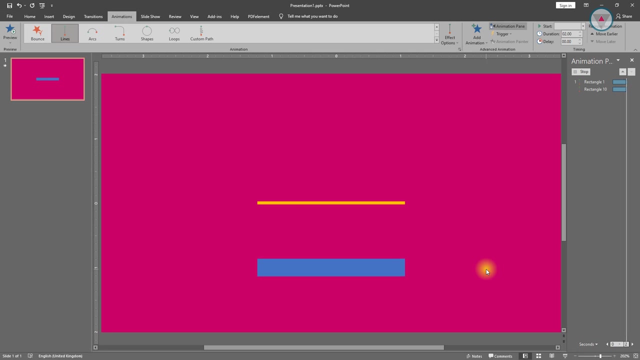 this to rectangle shape in the middle of this slide. after doing this, select this to rectangle shape and drag it to the left side. apply the lines animation. then select this rectangle shape and change its path direction to right and change its path direction to left. zoom out this slide by clicking here. then drag this endpoint and keep it in. 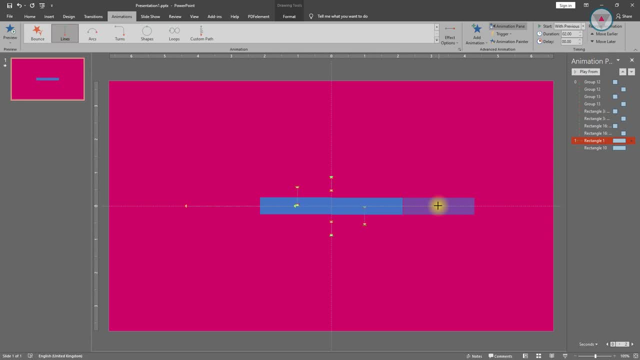 here and drag this endpoint too and keep it in here. then select these two animation and drag them. enable duration will be one second and select a start with previous go into the effect option and increase a smooth and duration. then select this animation and increase its delay one second. after doing this, select all of